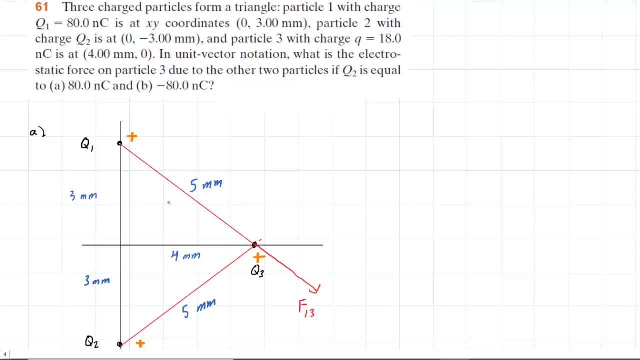 Now we look at the force that Q2 is exerting on Q3, and again in part A, Q2 is positively charged, so it too will exert a repulsive force on Q3 in this direction right here, and we can call that force F23,, symbolizing the force that charge 2 exerts on charge 3.. 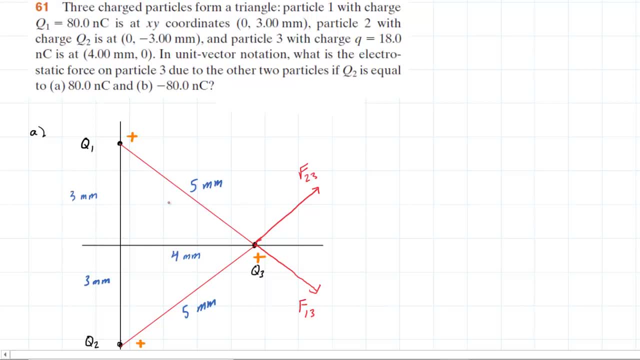 So that would be the completion of drawing in those two forces acting on Q3.. The next thing we would want to do here, perhaps, is to draw in the forces that are acting on Q3.. The next thing we would want to do here, perhaps, is to draw in the components of those forces. 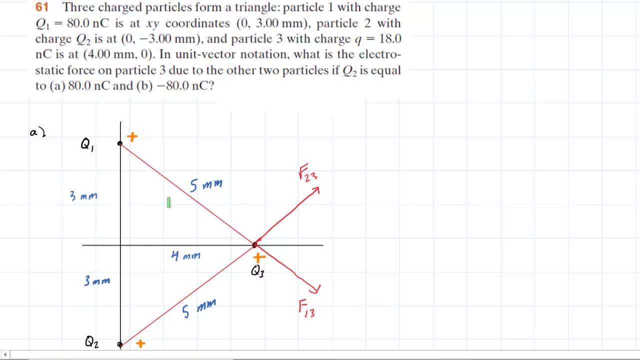 So let's consider the force labeled F23, and we're going to draw in the X and the Y components, And so for the X component, it would be projecting in the positive X direction. this way, We might call that F23X, just for now. 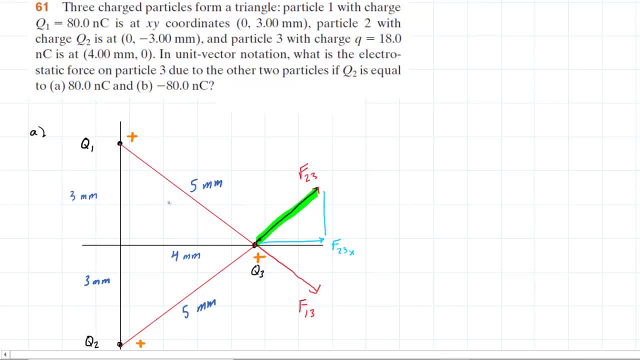 And then the Y component would be projecting upward in the positive Y direction. We can label that component F23Y And then we can see that there is an angle between F23 and the X axis. We might want to call that angle theta. 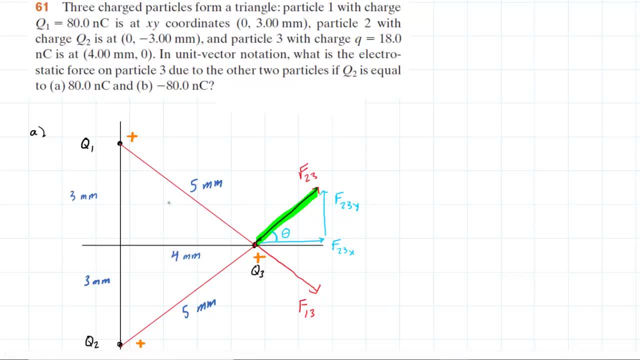 Now similar components can be drawn for the F13 force, So we would have- maybe we'll change colors here- we'll have- an F13X component going that way. It's going to get a little cluttered here, but we'll manage. 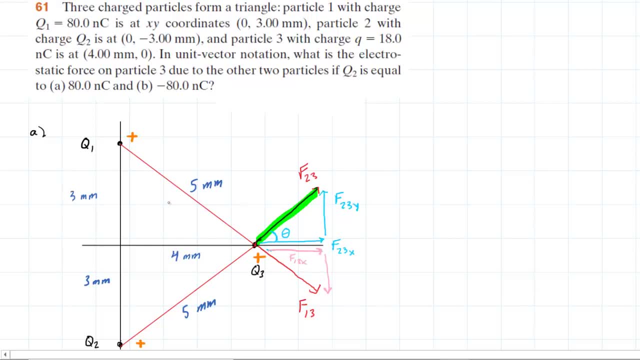 And then we'll have an Y component Pointing downward here. This can be F13Y. Now it's important perhaps for us to notice something special about these two Y components right here. Now we'll notice that the distance from Q1 to Q3 is the same as the distance from Q2 to Q3.. 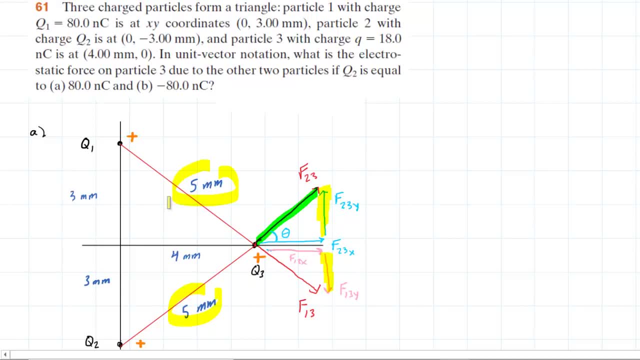 They're both 5 millimeters. We'll also notice that Q1 and Q2 are going to both have a a charge of 80 nanocoulombs, And so, since the charges- Q1 and Q2, are the same, 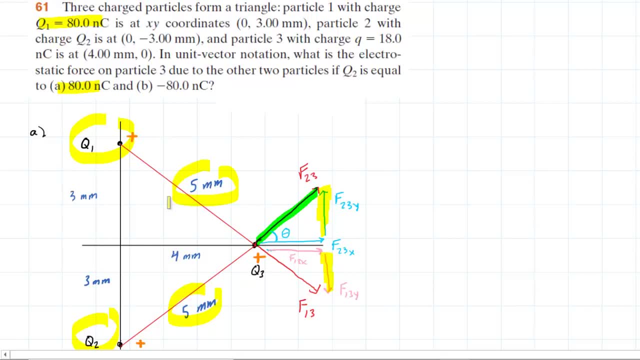 and since the distance from each charge to Q3 is the same, that means that the forces- the F23 and the F13, are going to have the same magnitude And therefore their Y components, one of which points upward, the other of which points downward. 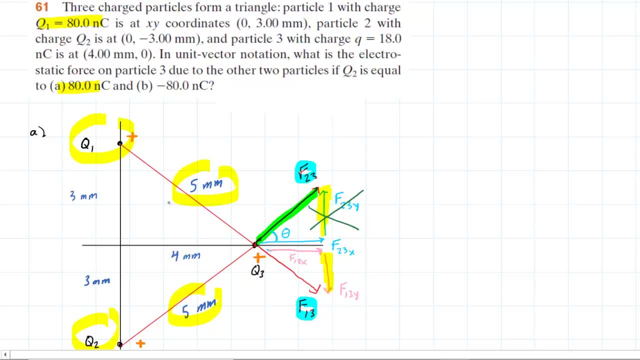 are going to cancel, So these Y components will indeed cancel out, leaving us only to worry about the X components. So it becomes our job to find the two X components, add them together, and that's going to be the answer to Part A of this question. 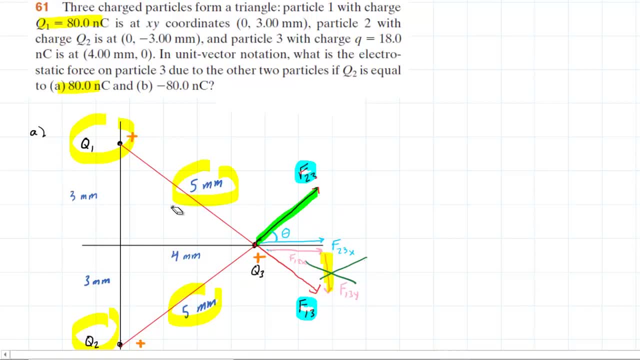 Perhaps we can even erase the Y components again, because they cancel out. We don't need to look at them right now. So the task is to find the X components. Hopefully we can understand too that the X components 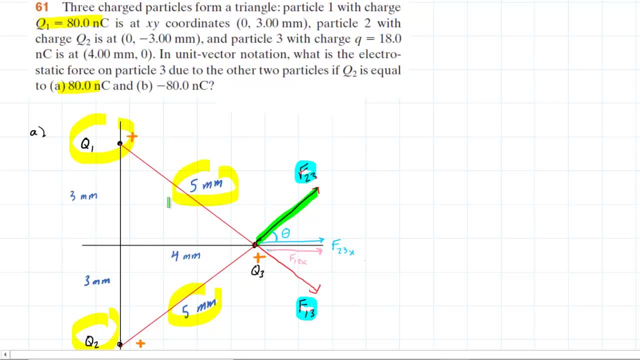 are going to be the same as well, because again, F23 and F13 have the same magnitude and this sort of angle here is going to be the same. So that angle right there will be the same as that angle right there. 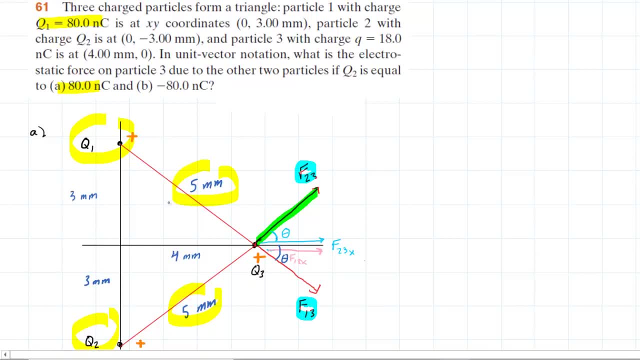 And so let's try to find the X component. It will be useful to get an expression for the X components. Let's consider a sort of right triangle that we can draw right about there. Remember, the X component is this: F23.. 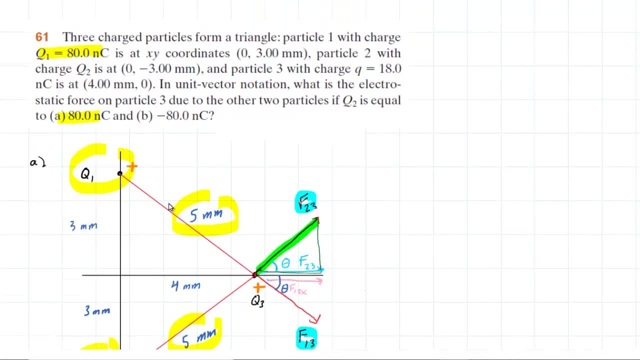 Remember the X component is this F23.. Remember the X component is this F23.. We can maybe shift it right there. Looking at that triangle, we might say that the cosine of that angle is equal to the adjacent side, which would be the F23,. 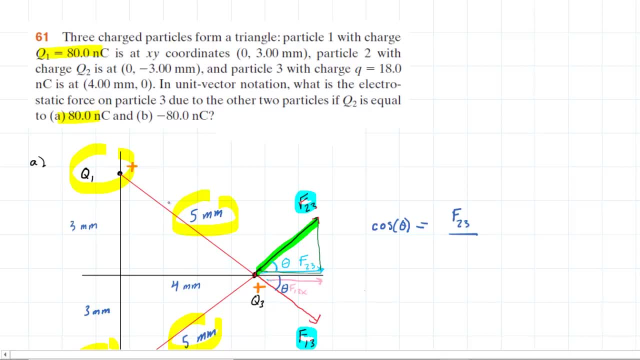 divided by, Or F23X. excuse me, That's the adjacent side of that triangle over the hypotenuse. Now, the hypotenuse is just this force in green right here. That's the F23 force. Now, it turns out, we can get a useful expression. 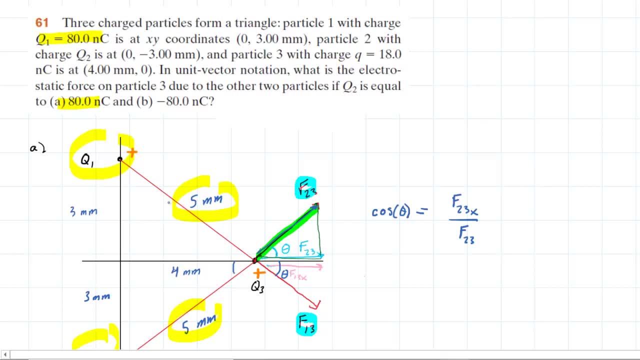 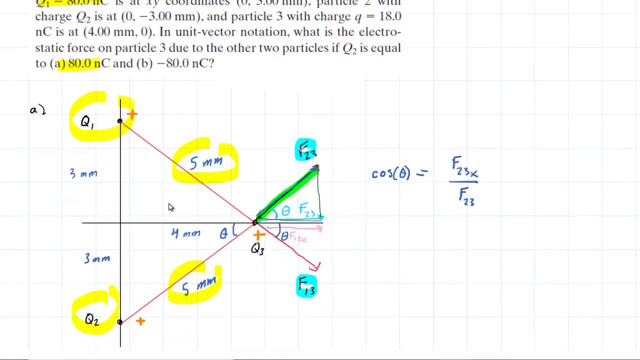 for the cosine of that triangle, for the cosine of that triangle, for the cosine of that triangle, We can use this theta here, which is identical to the theta in our triangle. And so if we look at this triangle right here, And so if we look at this triangle right here, 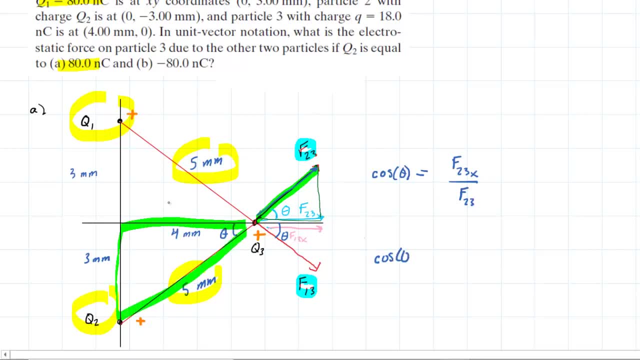 we can see that the cosine of theta is equal to the adjacent side of that triangle, which is four millimeters, divided by the hypotenuse of that larger triangle, which is five millimeters. The millimeters would cancel. So basically, the cosine of theta is four-fifths. 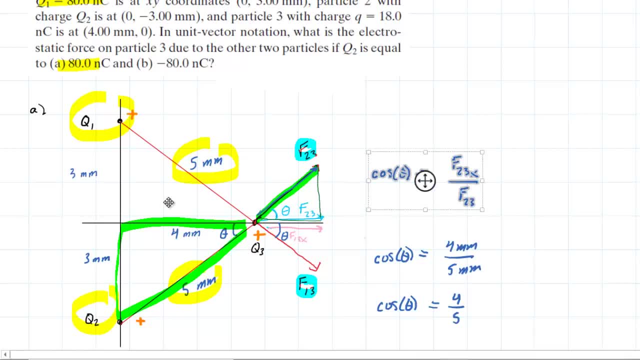 And this will be useful to us. Let's go back, then, to this equation right here, We now know that the cosine of theta is four-fifths, so we can plug that in, And again, what we wanna do is figure out an expression. 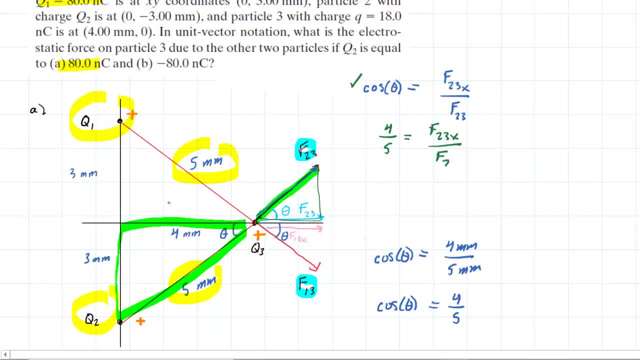 for the X component, And this will be pretty easy right now. We can just multiply both sides of this equation by F23.. These F23s will cancel out, And so we can now see that the X component of F23, if we kind of rewrite it here- 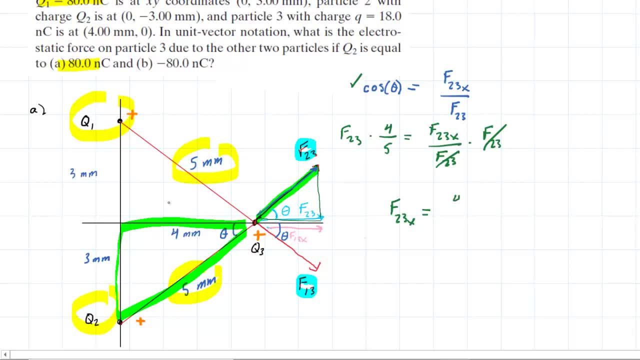 F23X is going to equal four-fifths multiplied by F23.. Now we can do better than this, because F23 is again the force between Q2 and Q3. That force is dictated by Coulomb's Law. 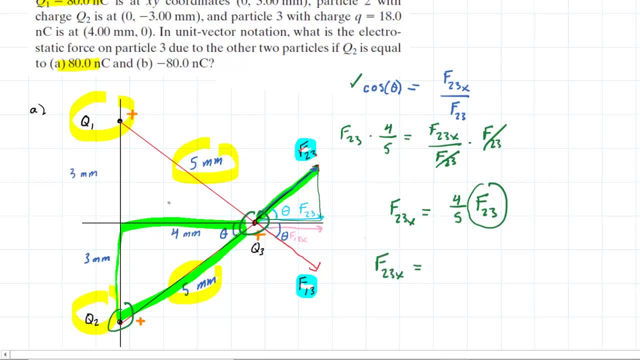 that we learned in this chapter. So we're gonna go in here and we're gonna use Coulomb's Law for F23.. Now remember, Coulomb's Law takes a constant, multiplies it by the magnitude of the first charge. 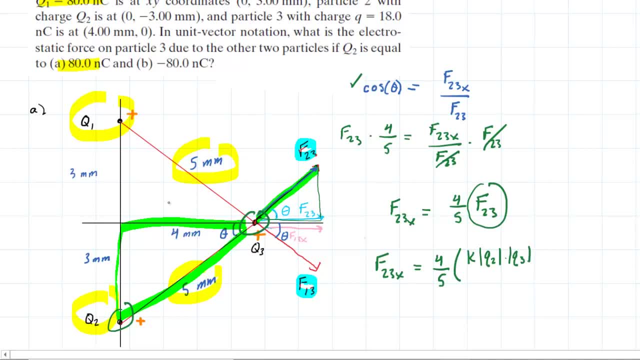 multiplies that by the magnitude of the second charge and then divides that by the distance between the charges squared. Now remember, here we know all these values. We can actually go ahead and find the X component by simply plugging in those values. 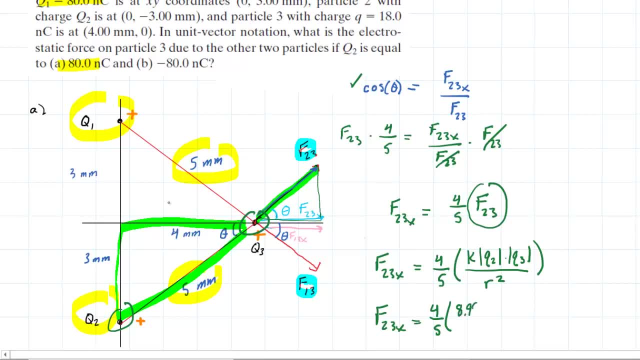 Now K is a constant. It takes on a value of 8.99 times 10 to the ninth. We will omit units right now for clarity. Q2 would be the charge on particle two, which for Part A is positive. 80 nanoCoulombs. 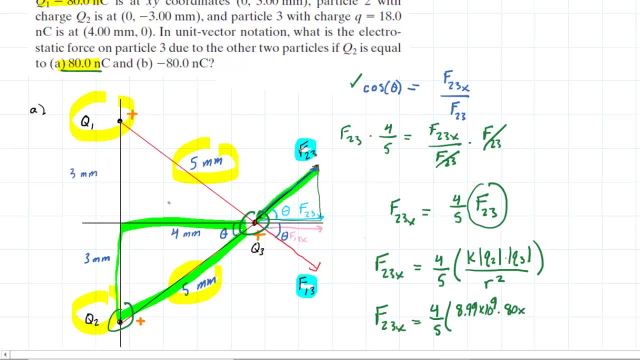 Now be careful here, because nanoCoulombs needs to be converted into Coulombs, and you do that by multiplying the 80 by 10 to the negative nine, So that would get that into Coulombs. now Q3 has a charge. 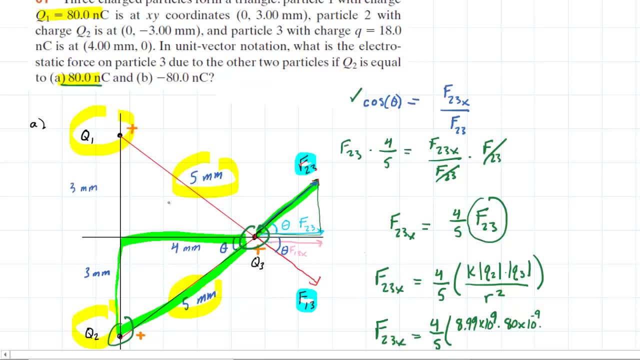 it has a charge of 18 nanoCoulombs. So we're gonna do 18 times 10 to the minus nine, and then we're gonna divide this by the distance between them squared Now, the distance between charges two and three. 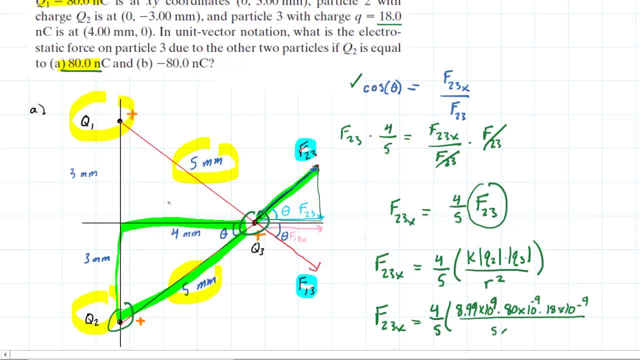 was the five millimeters. That's millimeters. so make sure you multiply the five by 10 to the minus three. That will convert that into meters. and then don't forget also to square that distance. So that's a pretty hefty calculation. 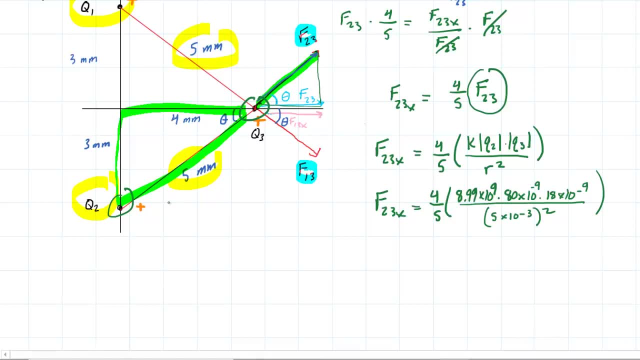 but if you punch that into your calculator you should end up with .414 approximately, And that's gonna come out in Newtons. So that's the X component of the F23 force. Recall that F13, this pink vector right here. 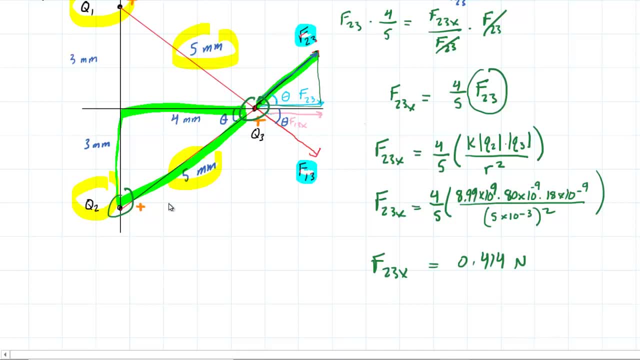 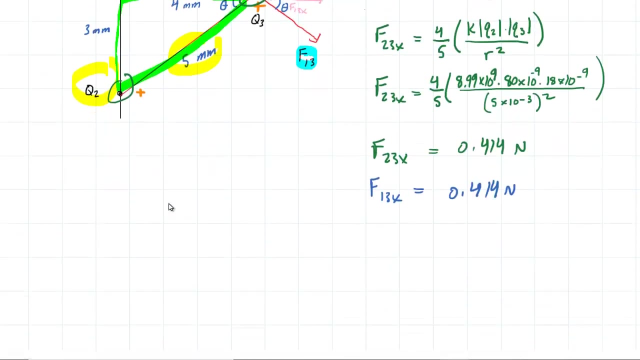 has an X component equal to F23.. So, without doing all of the math, we're gonna get to F23.. all of the math? we can simply say that f13 x component will also take on a value of about 0.414 Newtons and therefore, to get the net force acting on, 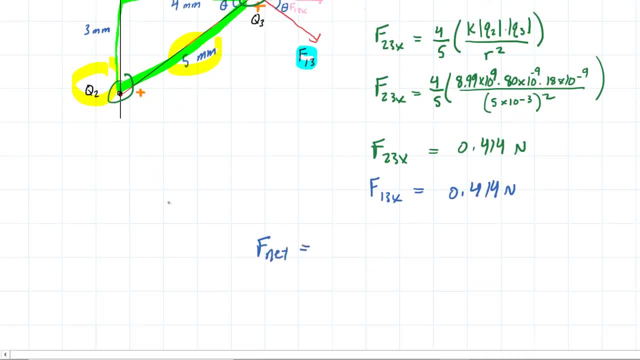 q3. we simply add these two x components together, so we're gonna have 0.414 Newtons plus another 0.414 Newtons. and because they want it in unit vector notation and because these are X components, we can just tack on a little. 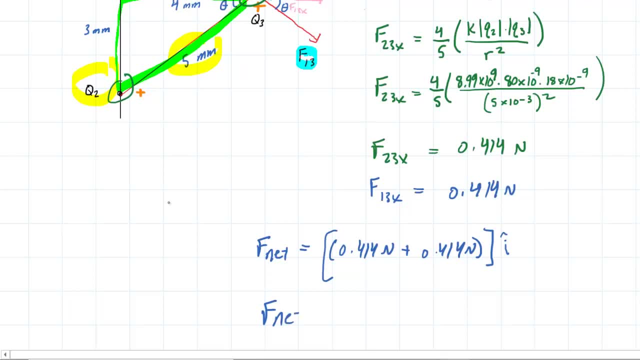 I hat here, I hat you recall, symbolizes the X direction, so we end up with about 0.828 Newtons and that will be in the I hat direction. there is no Y component recall so we don't have to write anything. I mean, if you wanted to you. 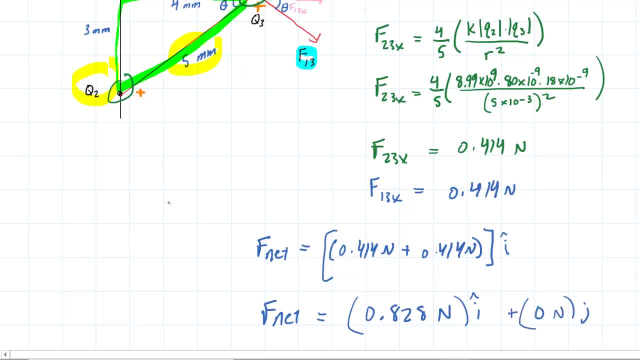 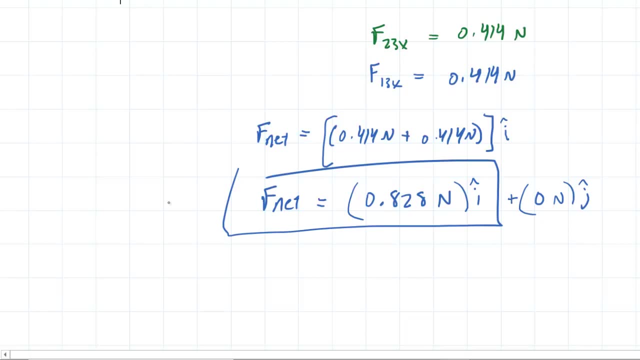 could say plus 0 Newtons, J hat. J hat symbolizing the Y direction, but really this is the best answer, right there. that's it for part a. let's set up part B now. for part B, the main difference is that q2 is now negatively. 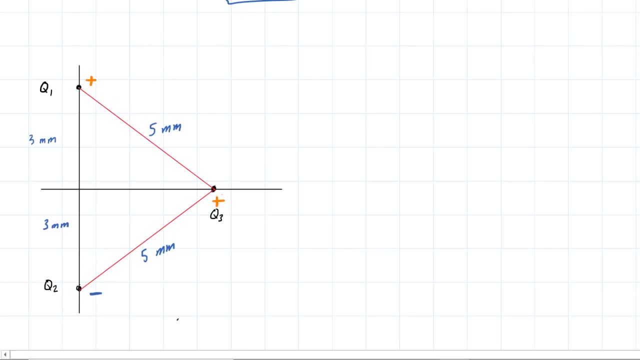 charged. so when we go to draw in the force that q2 is exerting on q3, instead of it being a repulsive force, this time it will be attractive, so we can draw a force pointing this way: this is basically q2 pulling on q3 towards. 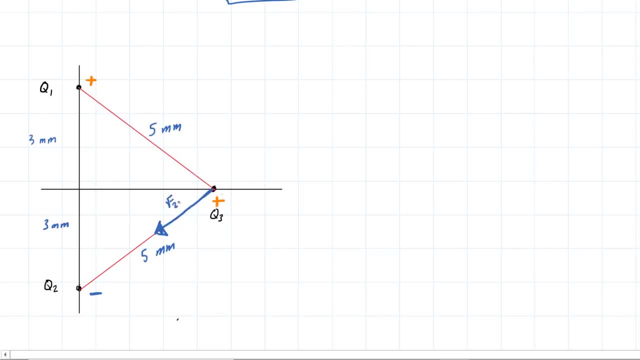 itself, this can be labeled f23 and the force is being pulled on q3. now this is So. that is an attractive force. The force that Q1 exerts on Q3 is still repulsive. They are still both positively charged, So we can draw that force going out this way and label that F13. 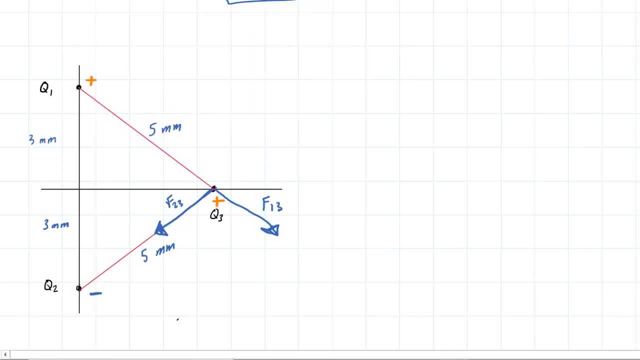 And then, as before, we need to consider the components of these forces. If we look at F23,, we would see that there is a Y component going this way. We can call that F23Y, And there's a component going that way. 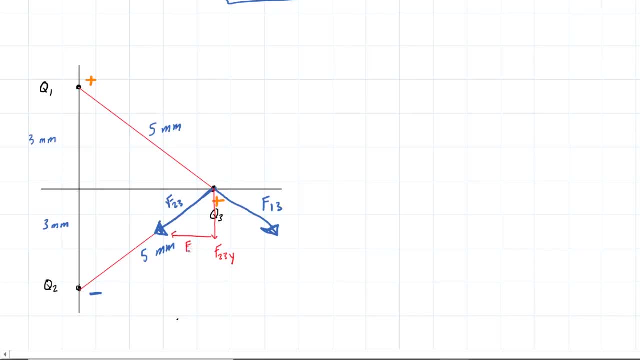 That is the X component, That will be F23X. We can draw the components for F13.. Similarly, there's a Y component pointing downward That's F13Y, And then there's an X component that points to the right. 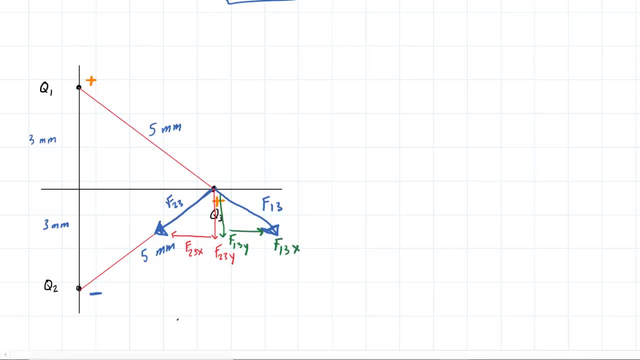 And that's going to be F13X. Now here's another secret to solving this question. Q1 and Q2 have the same magnitude. They're both magnitude 80 nanocoulombs- And then the distance to Q3 is the same for each of them. 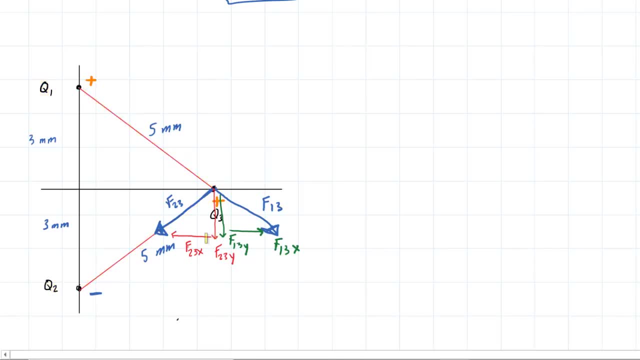 They're both 5. And so what this means is that the X and Y components are going to be identical in magnitude, And if you look at the X components, they point in opposite directions And therefore they will indeed cancel. So let's knock out the X components. 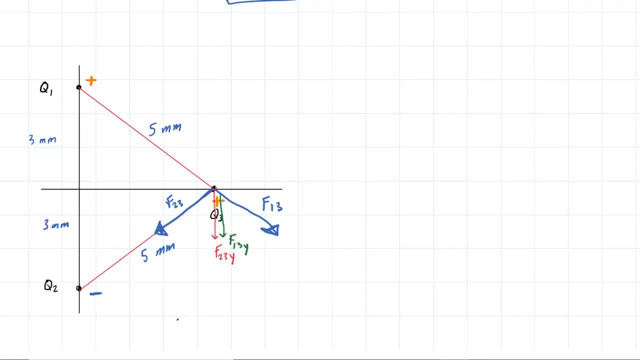 And we only need to concern ourselves with the Y components. So to find the Y component of, let's say, F23,, we can make a little triangle here, a little right triangle, just like this. And let's see Why don't we mark an angle? 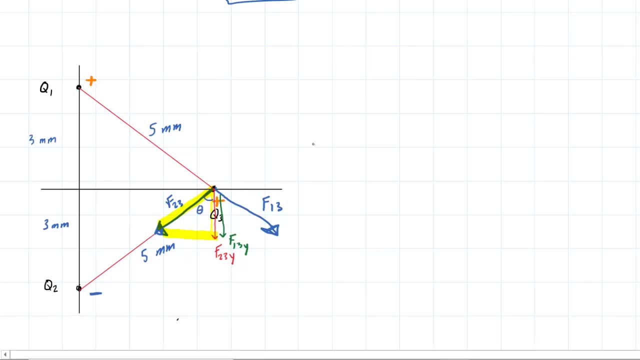 We can mark this angle here- We'll call that theta- And from that right triangle, which is a little bit messy, but we can say that the cosine of that angle will equal the adjacent side. Hopefully, from that yellow triangle you can see, the adjacent side is the F23Y. 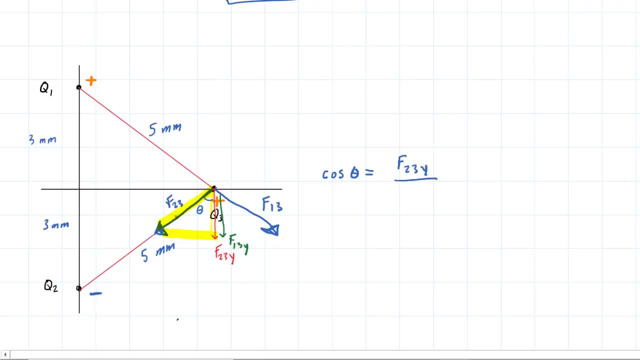 divided by the hypotenuse, which is just F23.. Now we've got to find an expression for the cosine of that angle, just like we did before, And it might be useful for us to sort of expand our triangle like this. We know that this distance was the 4 millimeters. 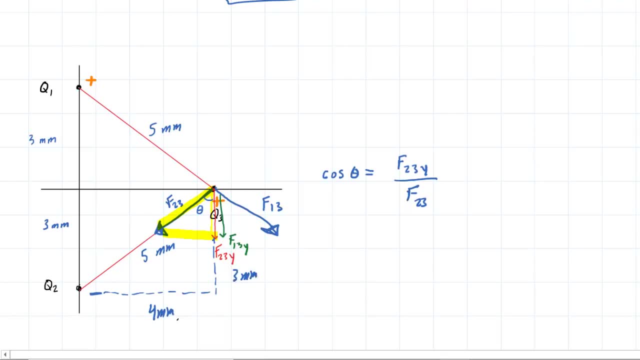 This over here is 3 millimeters, And then the hypotenuse is 5 millimeters. So right now we're looking at this larger triangle here, And so from that larger triangle we can hopefully see that the cosine of theta is the adjacent side. 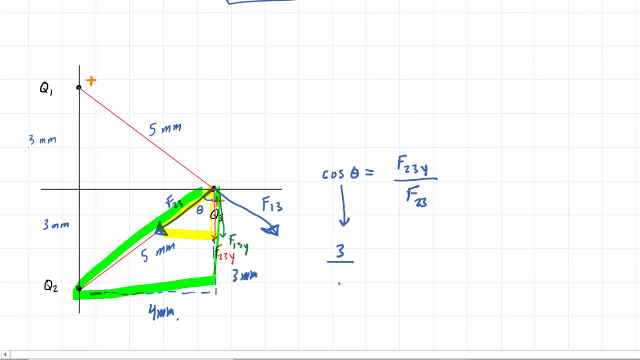 which is the 3 millimeters, divided by the hypotenuse, which is 5 millimeters, like that. Now we're going to solve this for the Y component. We'll just multiply both sides of the equation by F23.. 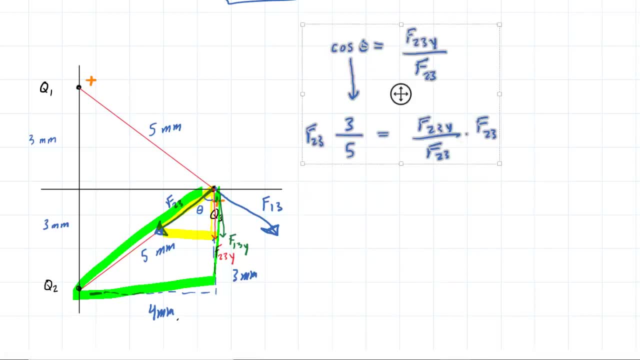 And we're going to pull this up, make some room. So now we have these: cancel. F23Y component is basically equal to 3 fifths times F23. And, just like before, we're going to substitute in an expression here for F23 using Coulomb's law. 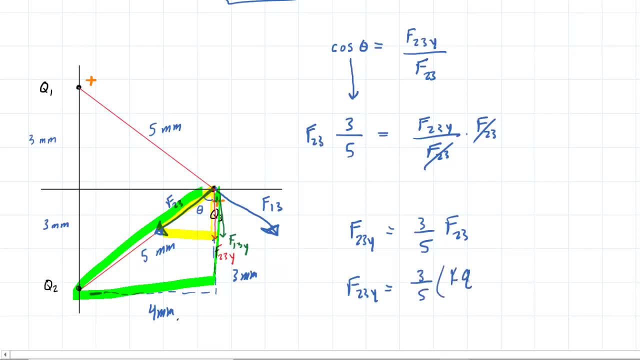 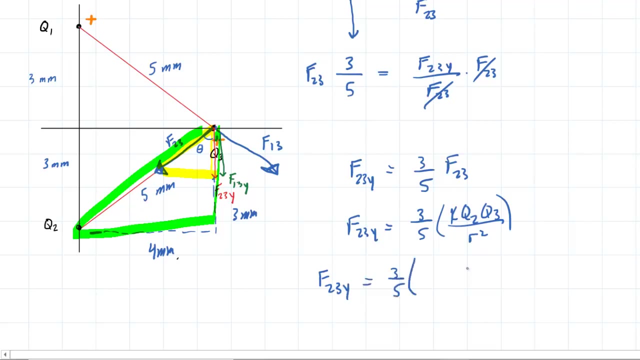 So this would be the constant K times Q2.. We can use the capital letters Times Q3 divided by the distance between them squared. Now we'll just punch in some known values to get this Y component for F23.. K, we know, is the 8.99 times 10 to the 9th. 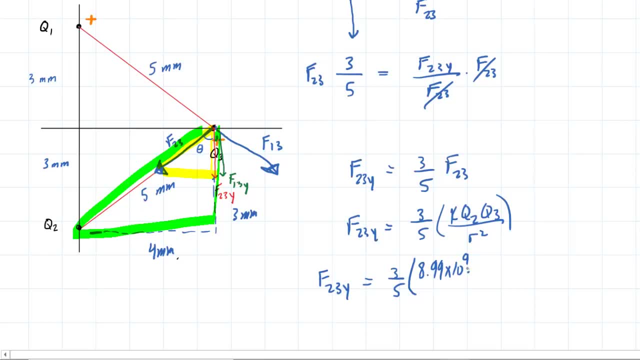 Q2 was now it was negative 80 nanocoulombs. But remember, we're just doing magnitude right now. These should have little absolute values on them, So you can see that You can still use positive 80. And then, for nanocoulombs, don't forget to multiply by 10 to the minus 9.. 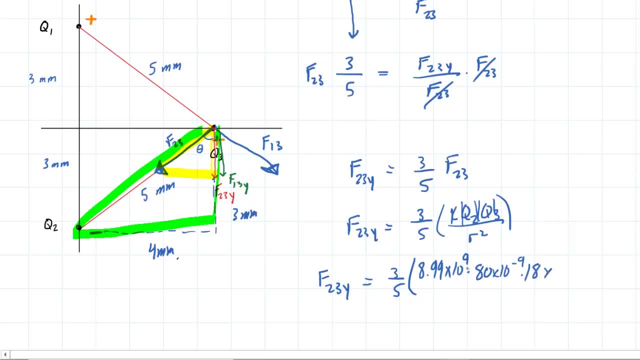 And then for Q3, it was 18 nanocoulombs. So multiply that by 10 to the minus 9.. And then divide it by the distance between them squared, which is the 5 millimeters. Don't forget to multiply the 5 by 10 to the minus 3 to get it into meters. 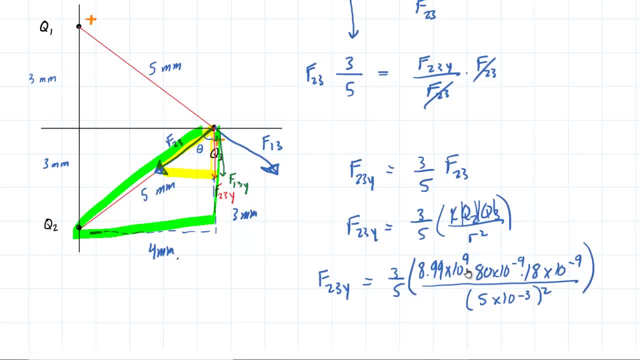 And then don't forget to square it. Let's go ahead and punch this into the calculator, And when you do that, you get the Y component of F23.. It's equal to approximately 0.31.. 0.7, something like that. 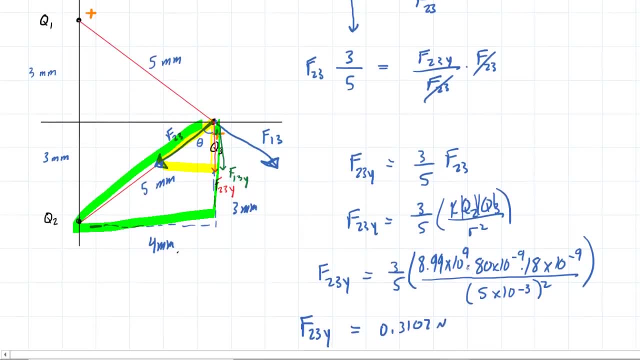 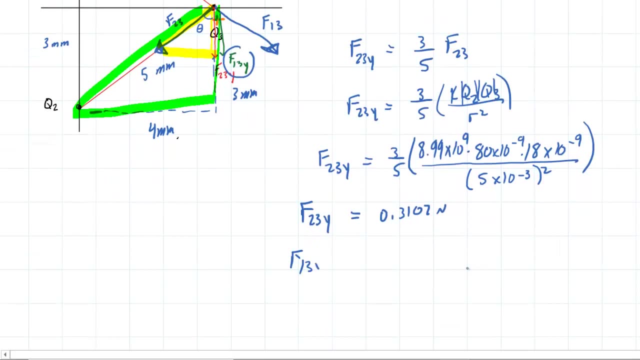 That'll be in newtons. Now. let's not forget that the Y component for F13 was the same, So we also know that F13, Y component is the same value. So to get the net force, we're going to add them together. 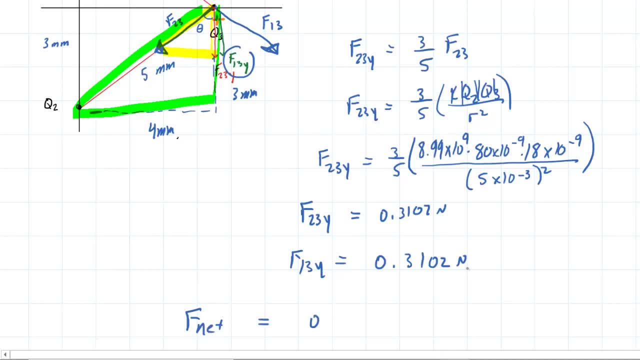 Now, if you add those together, you get about 0.621.. This is in newtons, But let's be careful. Look at the direction of the Y components. It's as messy as this This picture is. the Y components are both pointing downward. 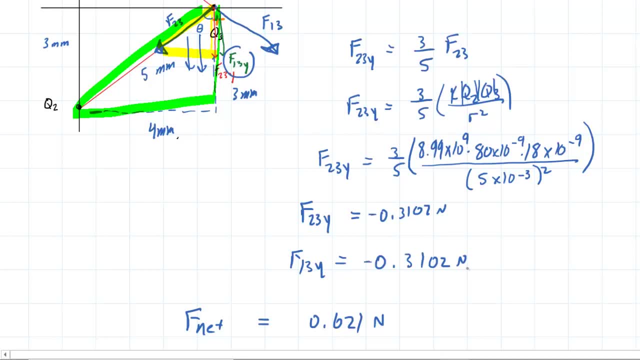 So the truth is, when we added these, we should have put little negative signs on these guys, because they're both pointing downward. Therefore, this should have a negative sign on it. And to complete the unit vector notation, this will be J hat, which symbolizes the Y direction.